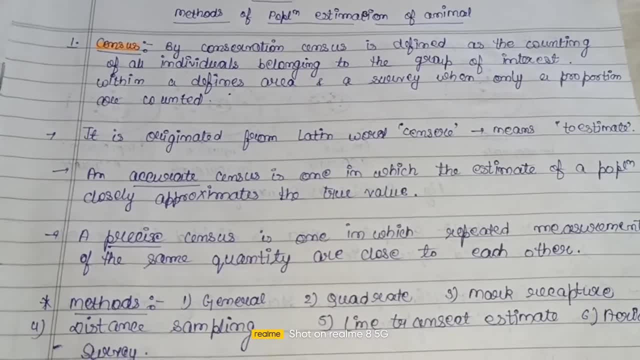 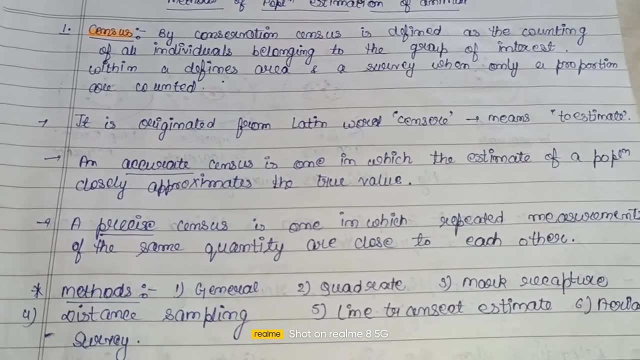 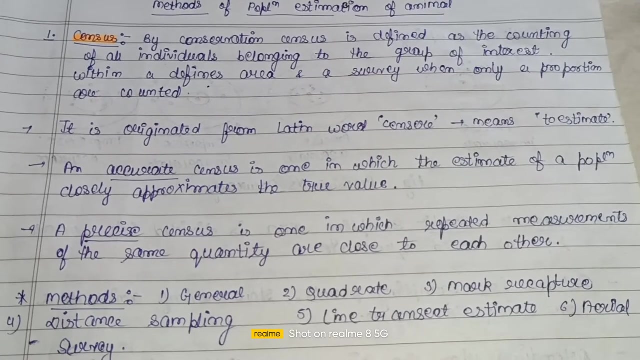 value, That is, we can say the degree of closeness, is noted here. Then a precise census is one in which repeated measurements of the same quantity are close to each other. That is precision refers to how close measurements of the same item are to each other. So we can say the precision. 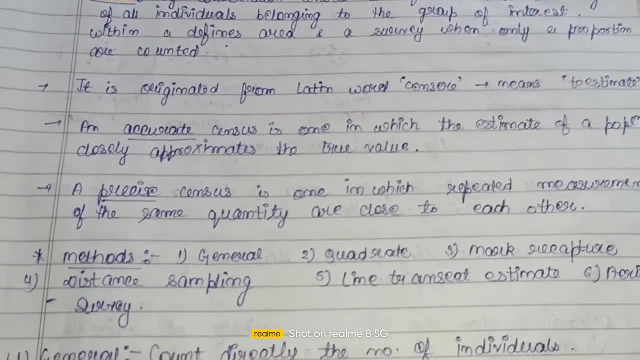 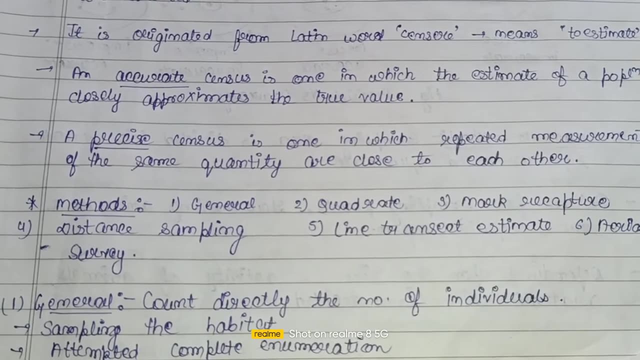 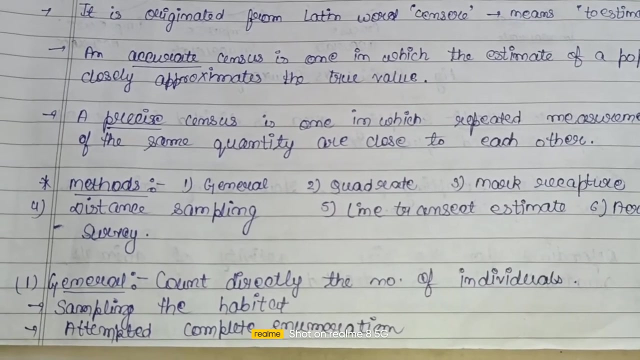 and accuracy are independent of each other. Methods under the census are: first is the general method, then quadrate method, mark recapture method, distance sampling method, line transact estimate and aerial survey. So first is starting with the general method. So here count directly the number of individuals. 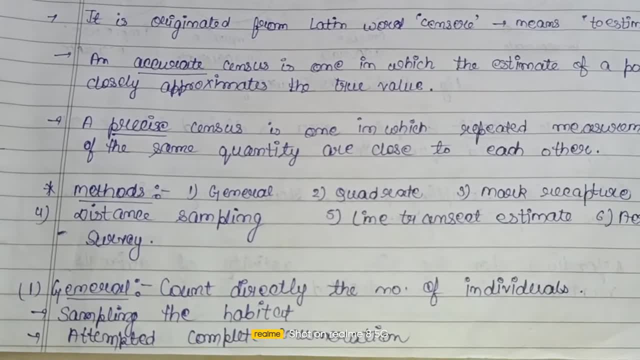 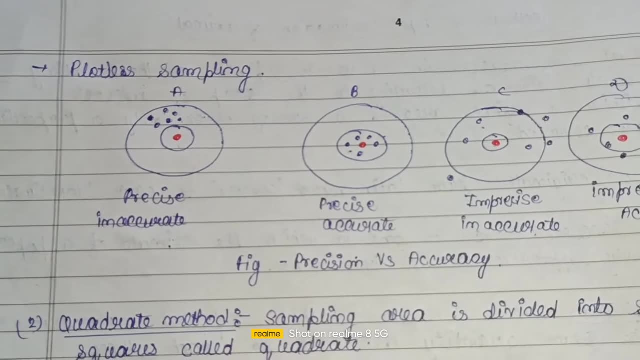 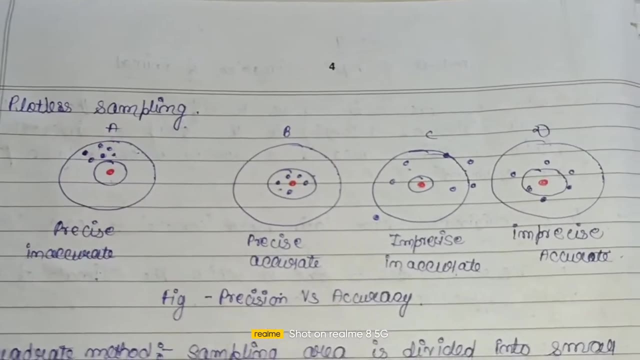 Then start sampling the habitat in which an animal lives and attempt the complete enumeration, that is, the counting and plotless sampling That is here. we should not use any types of quadrate method. Okay, So the difference between precision versus accuracy is shown in this. 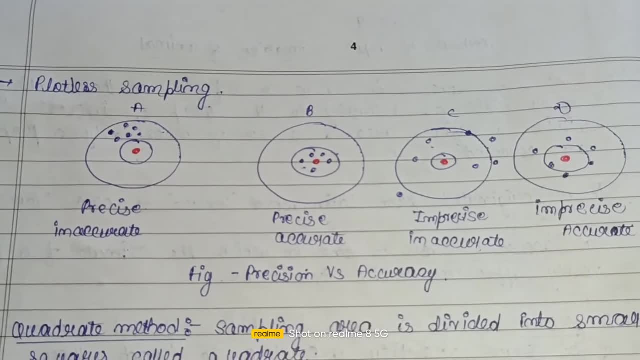 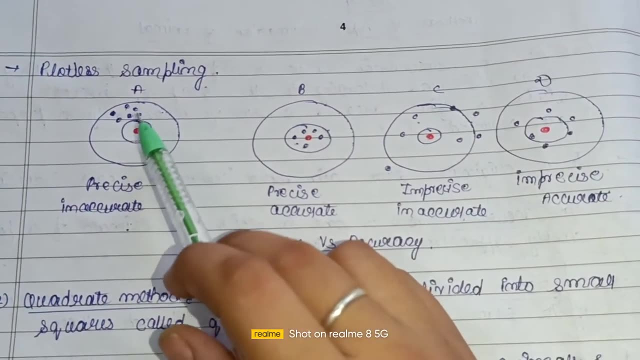 diagram. So accuracy generally means that we can say that near to the true value measurement. So suppose this is our target, The main center is our target. So here the values are not close to the target, so it is inaccurate. Then again it is the values. 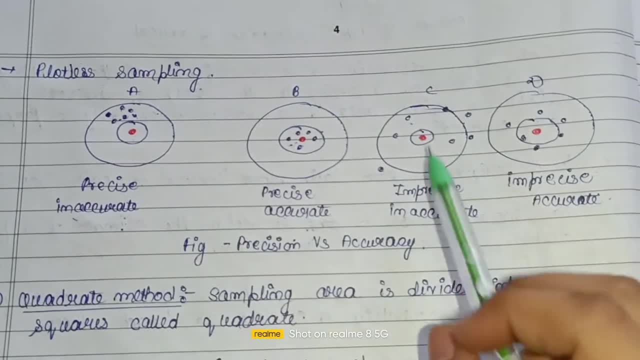 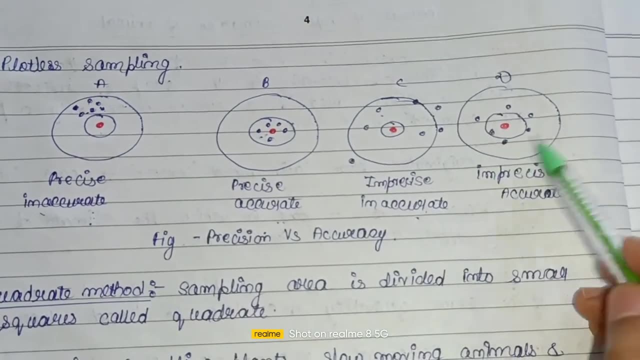 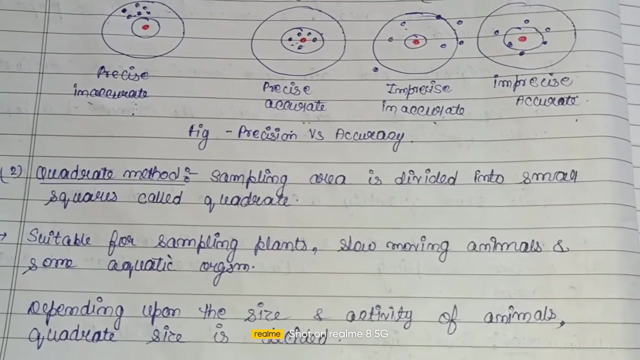 are closer to the target, so the value is accurate. Then again, these are not closer to the target, that is, they are far away, so that they are inaccurate. and they are somewhat near to the target, so they are again accurate. So now the quadrate method. So sampling area is divided into. 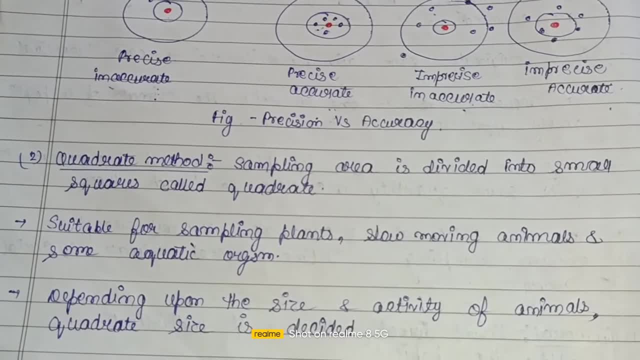 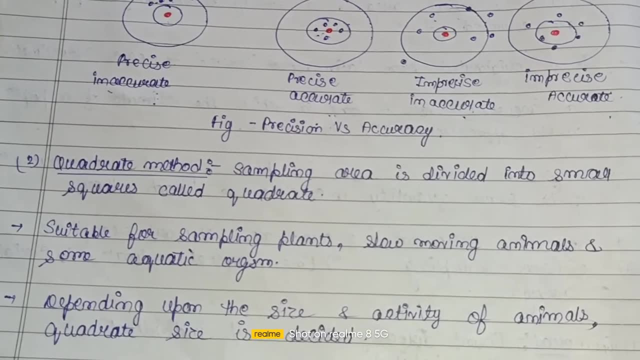 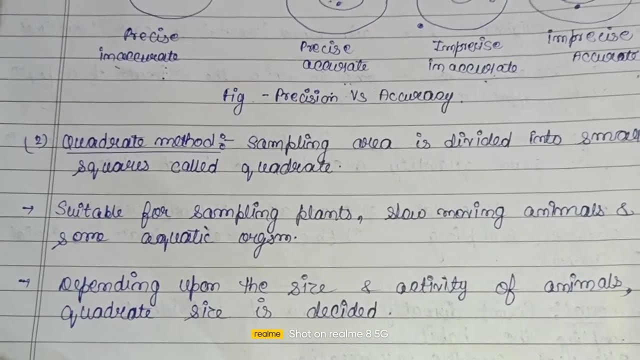 small squares that are called quadrate. It is suitable sampling plants as, because they lack the locomotion, slow moving animals and some aquatic organisms. so, basically, why we are considering this? because, so, as in case of the plants, they do not, they are not able to change their place because they lack the locomotion. 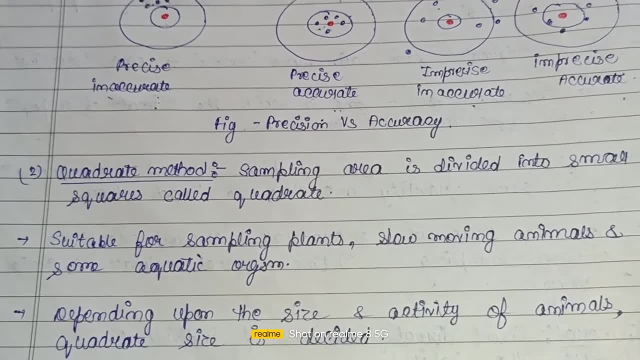 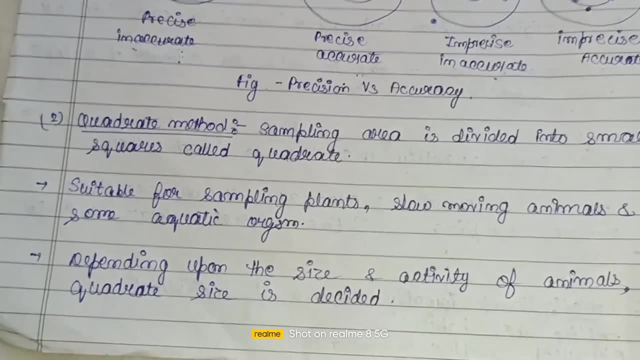 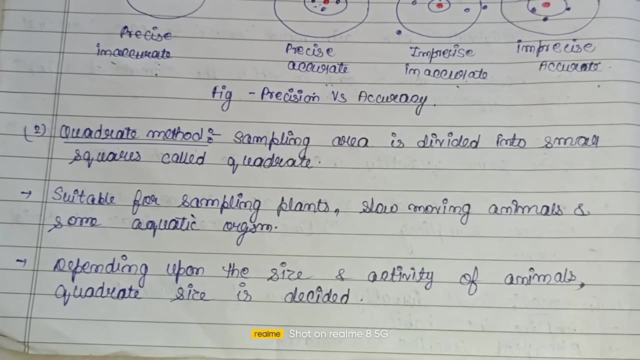 feature. or in case of the slow moving animals, they cannot travel much as compared to the faster animals, so this method is suitable for them only. so, depending upon the size and the activity of the animals, the quadrant size is decided. so this is a diagram representing the quadrant sampling. 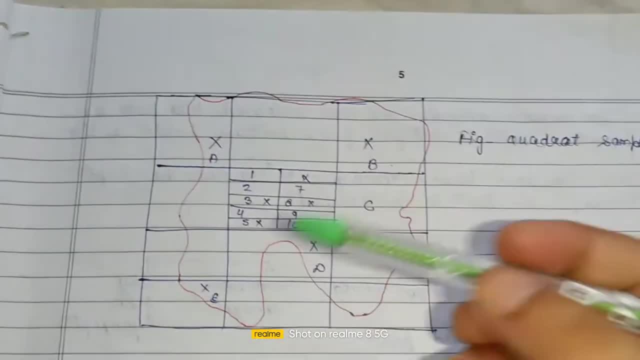 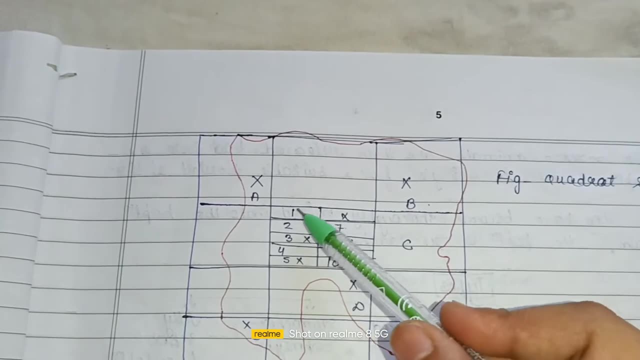 method. so here we have marked basically four quadrants, that is first a, b, c, d and e, and here in a, one single quadrant, we we have observed one species, then seven, then three, eight simultaneously. so we have observed one species, then seven, then three, eight simultaneously. so we have observed 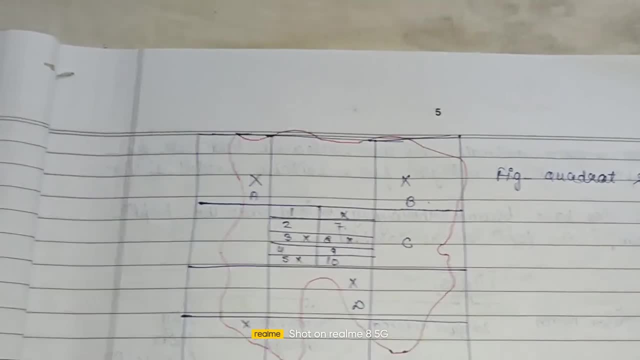 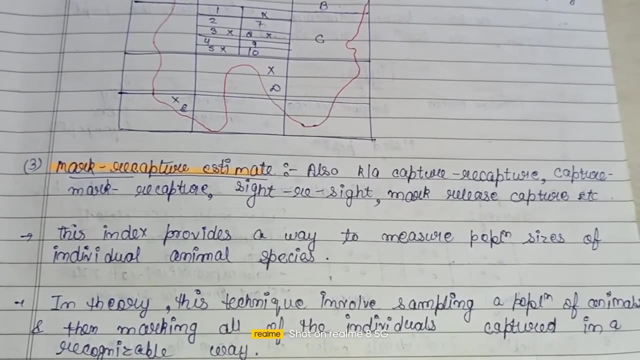 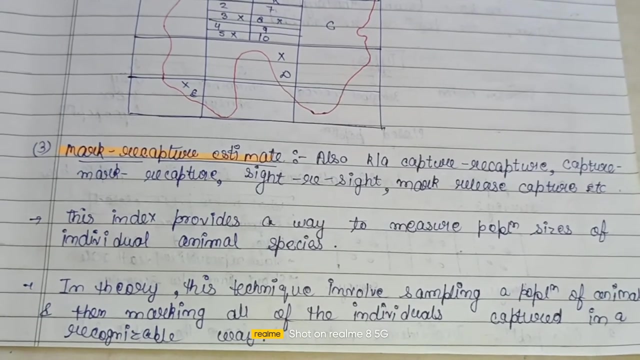 So by this method we can estimate the population of a particular animals. Then a third is the mark recapture estimate, So it is also known as capture recapture, capture, mark recapture, site recite, mark release capture, etc. 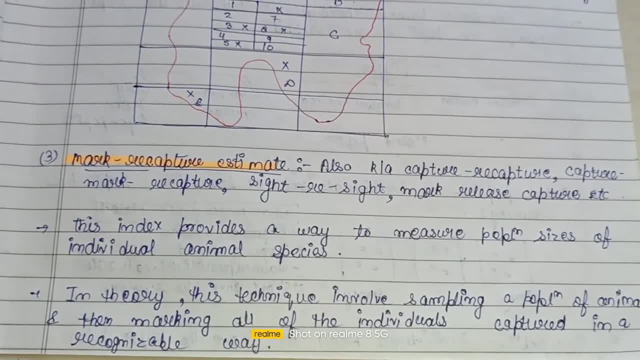 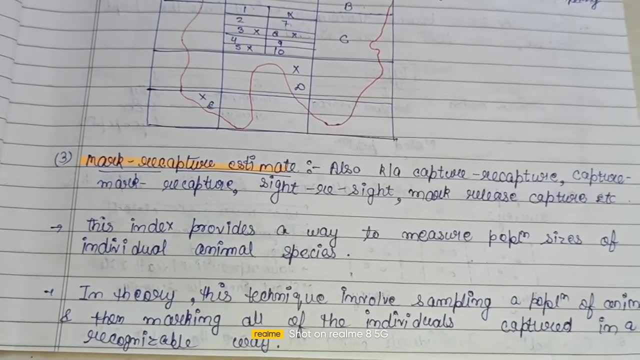 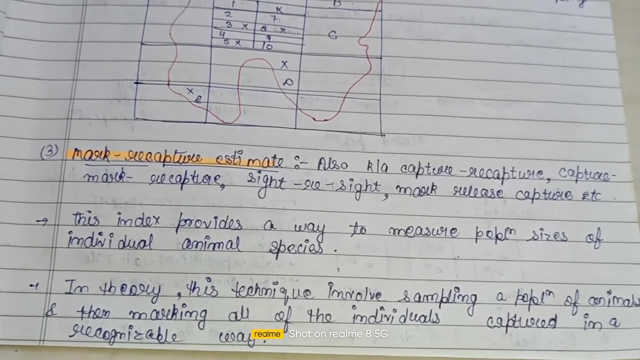 So it is known by various names. This index provides a way to measure the population sizes of individual animal species, That is, individual animal can be. population estimation can be done here In theory. this technique involves sampling a population of animals and then marking all of the individuals captured in a recognizable way. 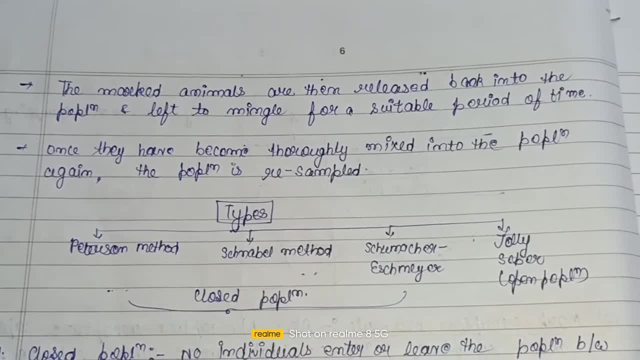 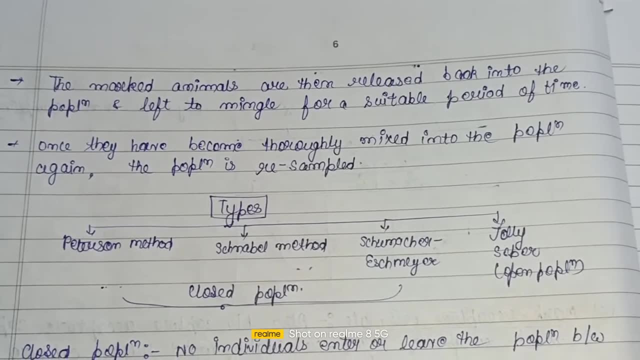 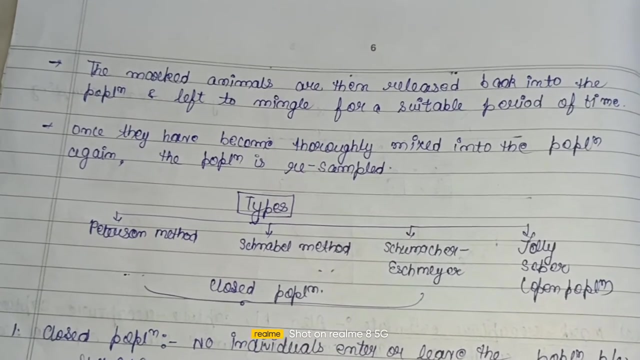 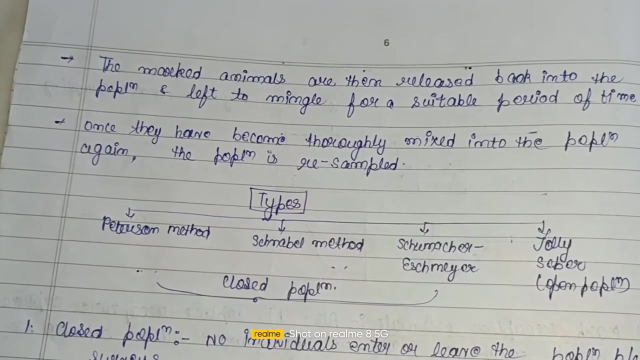 So the marked animals are then released back into the population and left to mingle for a suitable period of time. Once they have become thoroughly mixed into the population, again the population is re-sampled, So it is known by various names. So what basically happens here is that we generally tag an animal by a mark and then left it in its habitat and again count it after a suitable period of time. 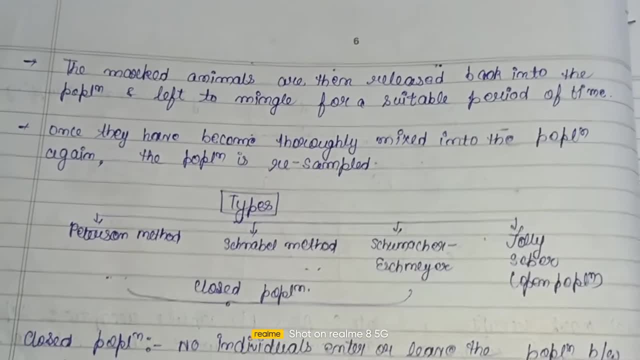 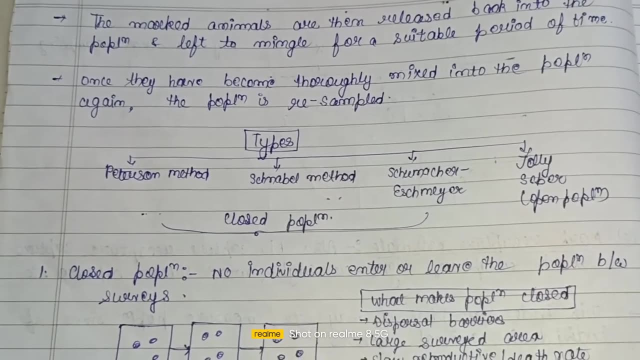 So, basically, mark recapture method includes this type of process. There are various types of methods through which this process should be completed. First is the Peterson method, then Scnabel method, then Squantmatcher Eschmeyer method and the Jolly Sober method. 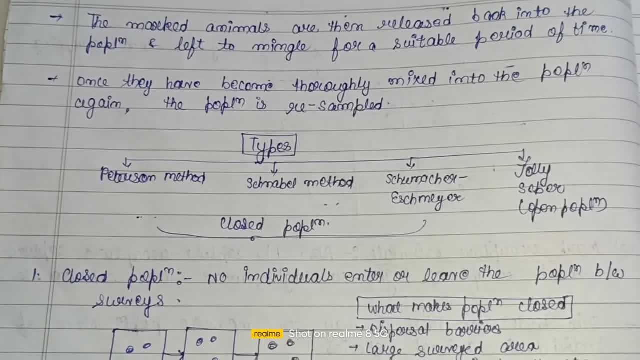 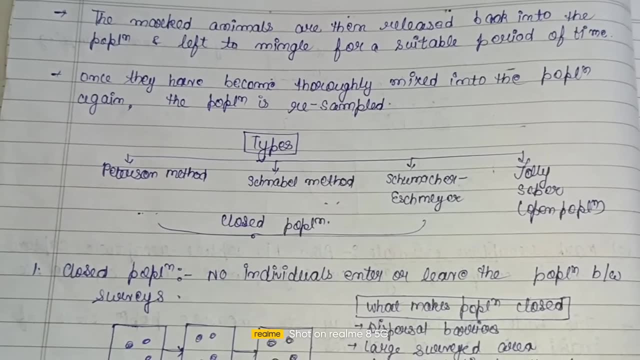 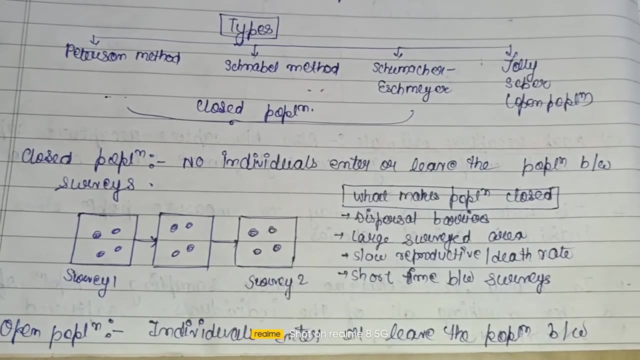 So basically first three are done in a closed population and the last one is done in an open population. So first we have to understand what is a closed population and what is an open population. So closed population: No individuals enter or leave the population between the survey. 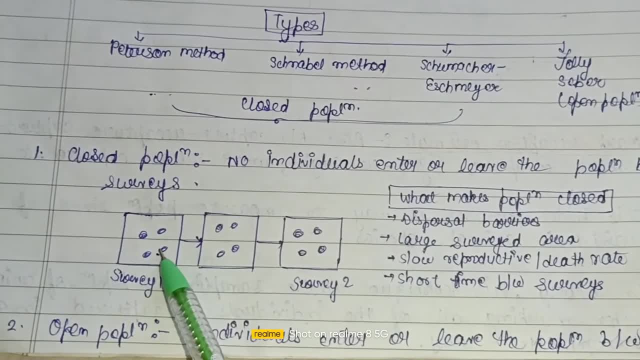 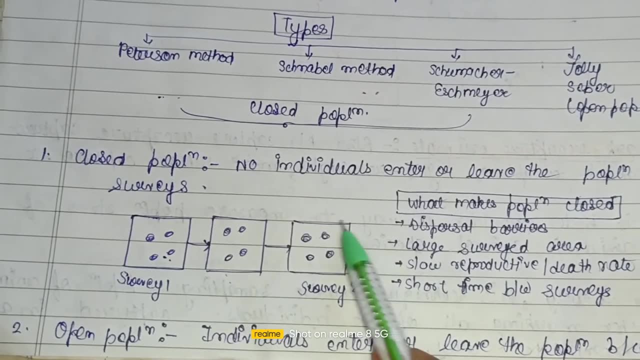 That is, this is the first survey. We have marked the animals. Then after that, for some sort of time, the animal do not leave that place, And also during the time of the survey too, also that animal do not leave that particular place or habitat. 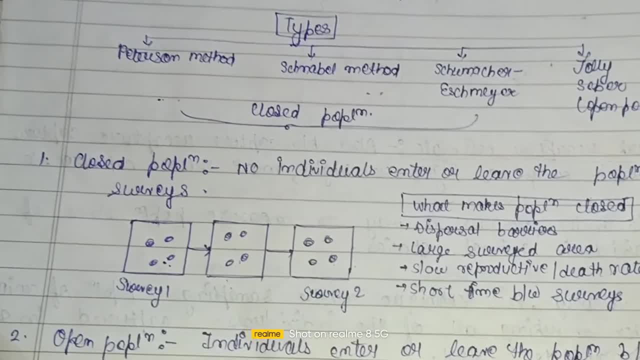 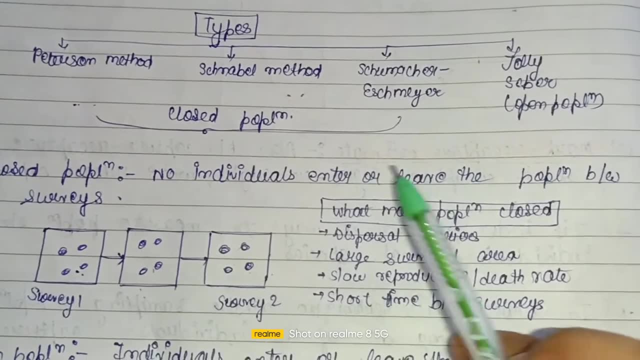 So this is a closed population where animal do not leave its natural habitat. So now the question is: what makes a population close? That is, what are the factors behind it? So first is the dispersal barrier, That is, if some sort of geographical barrier was there. 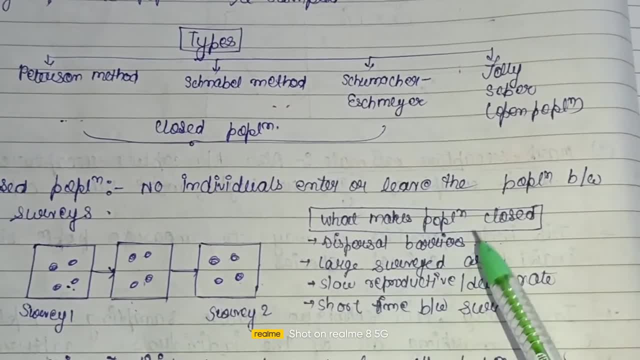 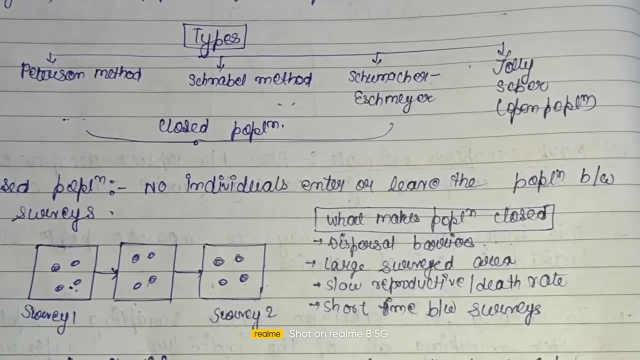 So there was a problem in dispersal of the particular population so that they remain confined to a particular area, only Then large surveyed area. That is, if we survey a very large area, that only if animal move. it moves only to a particular distance only. 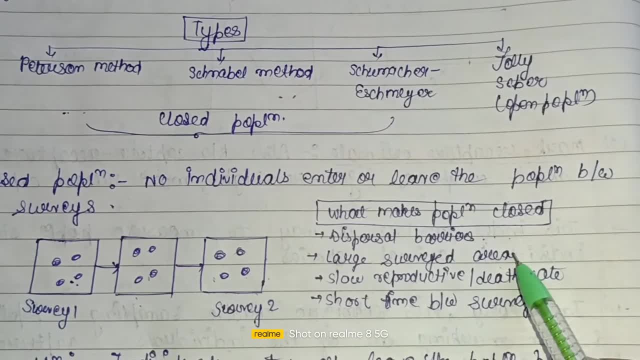 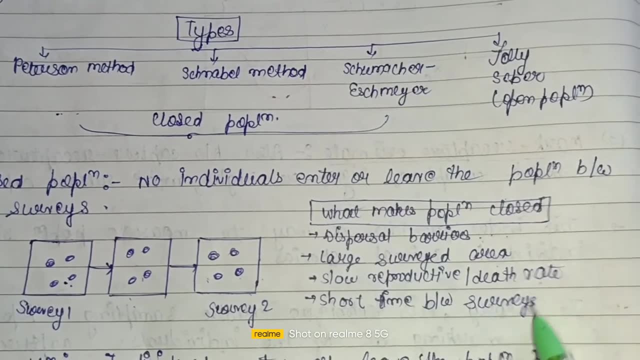 That is only a large distance So we are able to calculate that easily. Then slow reproductive or death rate if animal have, And the short time between the survey, That is, if we decrease the duration between the time of the survey, between the survey 1 and the survey 2,. 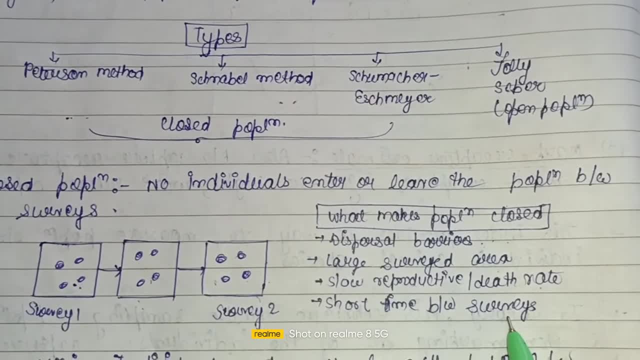 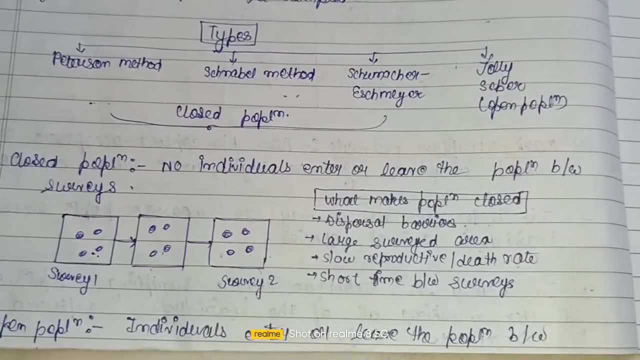 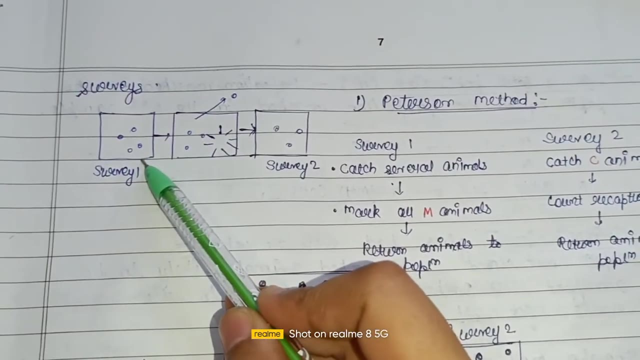 we can easily capture or we calculate the values according to the capture, Then recapture method, Then the open population. So here individuals enter or leave the population between the surveys. So in survey 1,, as we can see, 4 individuals were there. 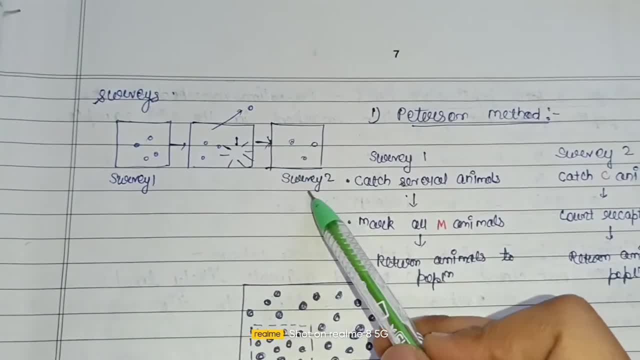 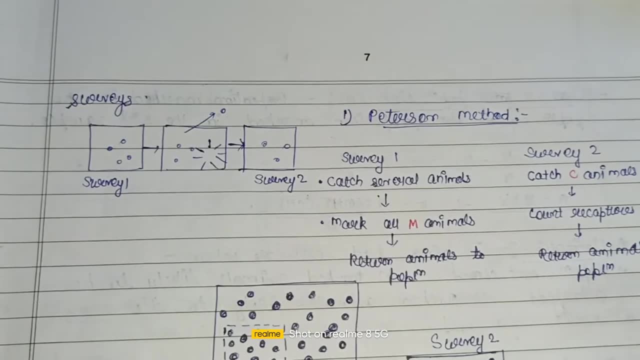 But between that time 1 left its place and again in survey 2, that is, only 3 were remaining. So this is a condition for open population. So first method is the Peterson model. So here in survey 1, we catch several animals. 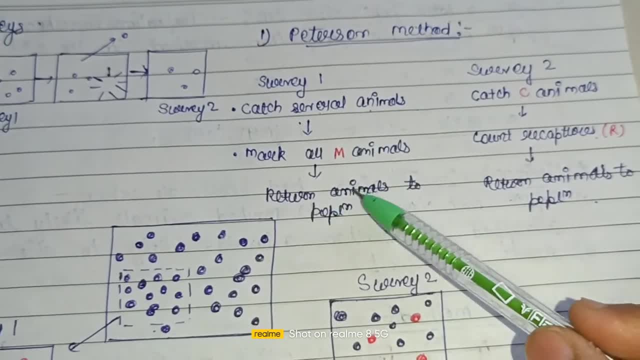 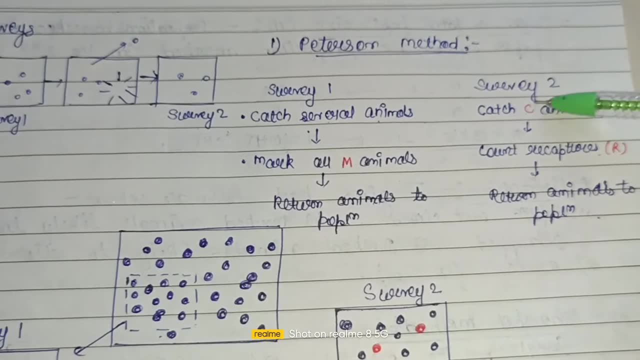 Then mark all the animals by M and then return animals to the population After that. in survey 2, we catch C animals, that is, denote them by C and then count recaptures, That is, recaptures are those that are counted here as M. 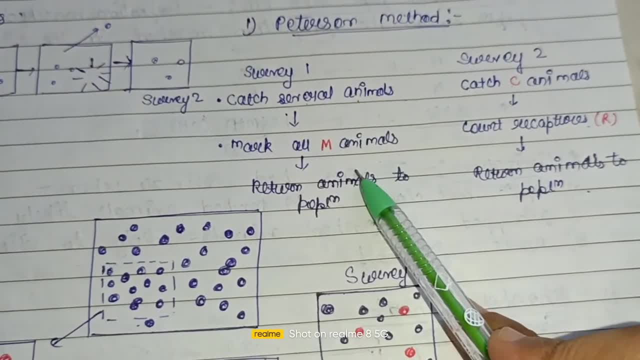 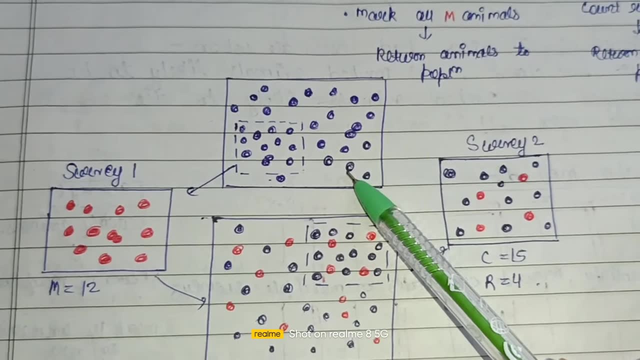 That is, they are denoted as R, that is, from this population also, and then return animals to the population again. So this is a diagram. This was the original source of population, from where in survey 1, mark capture. 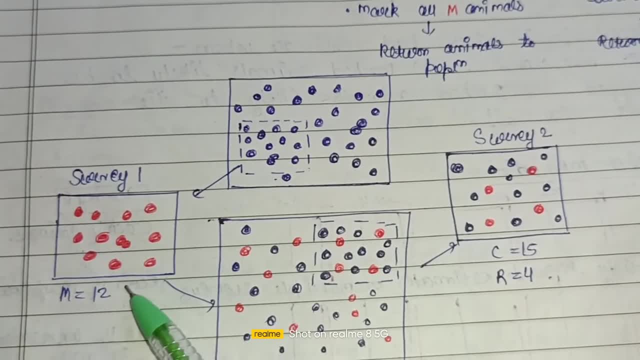 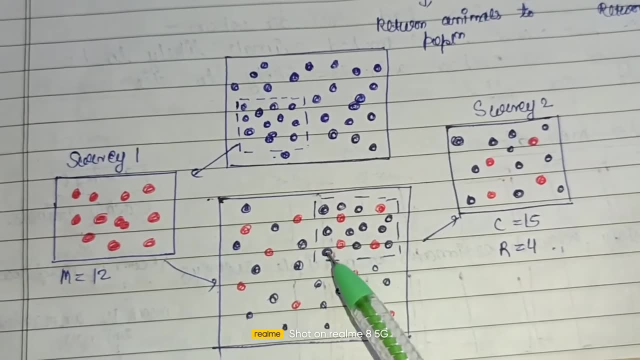 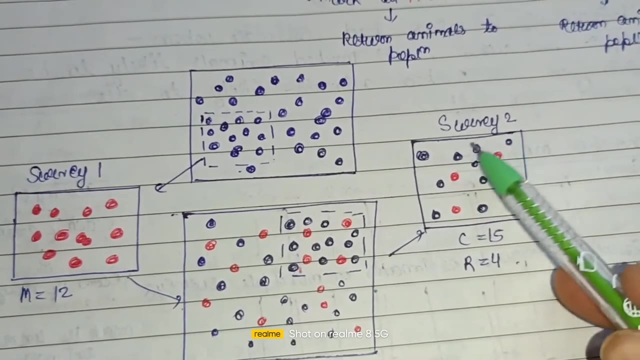 capture, animals are taken up. That is, M represents the 12. Then again they are left into their natural habitats for mingling up, That is, they mix up very well with others. And again in the survey 2, we captured, that is again with mark 15, that is new one. 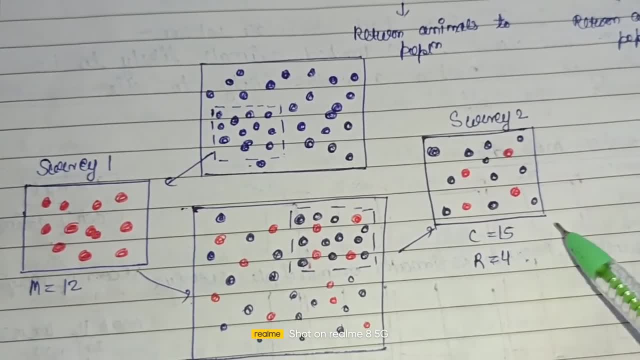 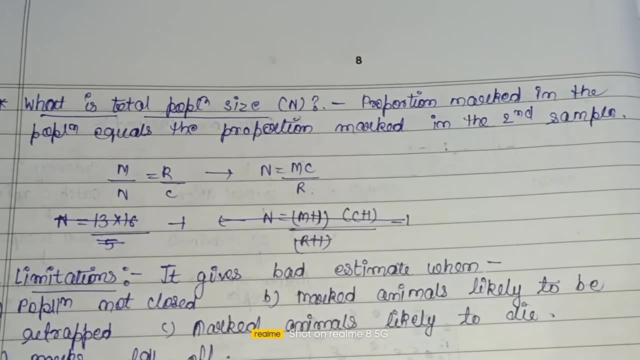 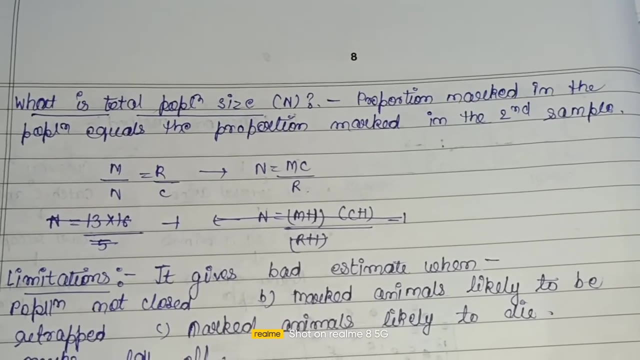 And recaptures are 4, that is, 4 are those animals which are previously counted in that survey. So they are the recaptures one. So what is the total population size? That is capital N here. So the proportion mark in the population, that is the total population, equals the proportion mark that is in the second sample. 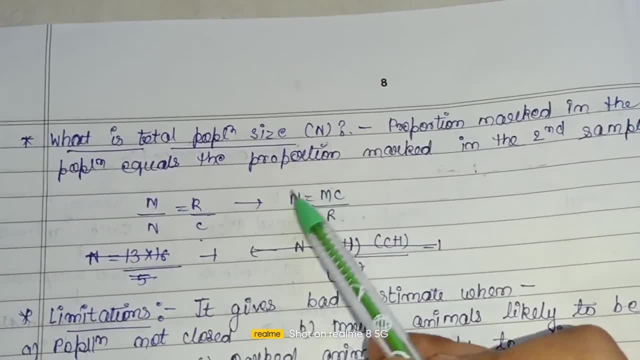 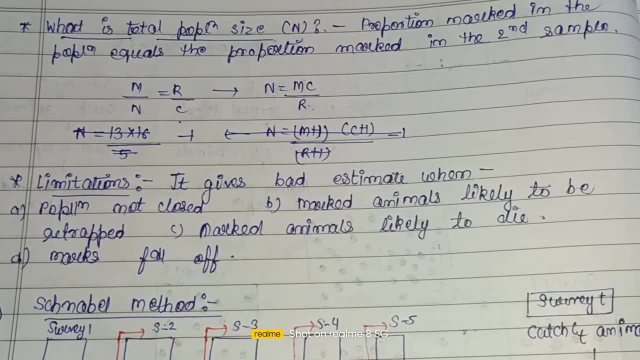 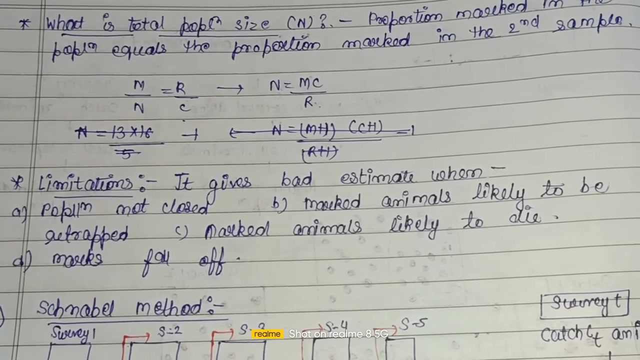 So this is the formula M upon N, R upon C. So N is equal to MC upon may R. So there are some sort of limitations in this method. First is it gives the bad estimate when, then, certain conditions are. first is, the population is not close, that is, when an animal moves from one place to another. 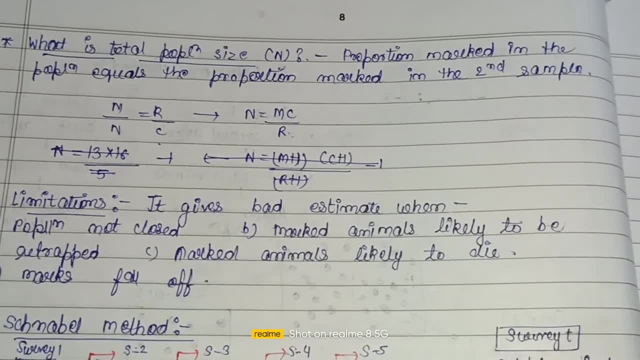 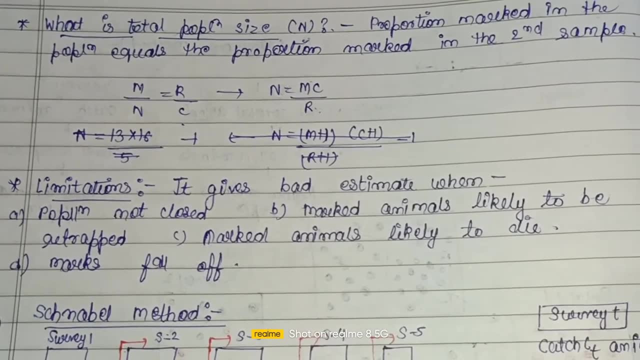 the condition is not fulfilled, then the marked animals likely to be re-trapped. that is there. there is a chances that they should be recaptured. yeah, that should be there. and the marked animals are likely to die. that is, they should die, and also the marks follow. so the accurate value is: 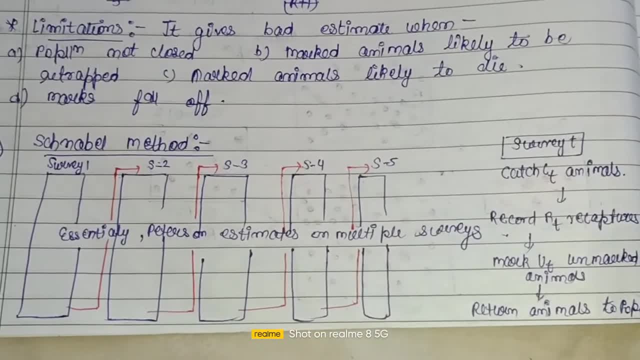 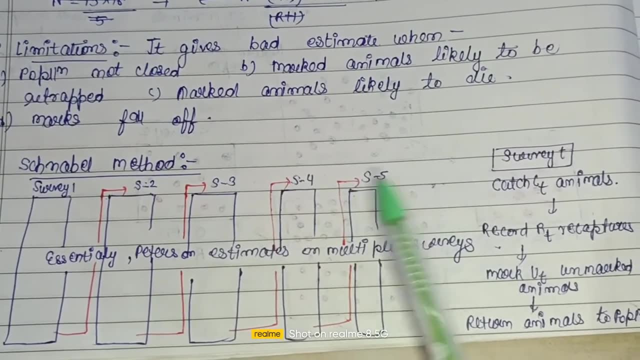 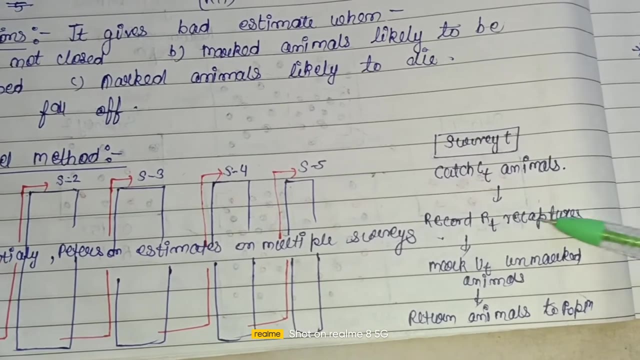 not observed. here then again is the scnable method. so in this method also various surveys are done, that is survey 2, survey 1, 2, 3, 4, 5 and simultaneously so survey, that is t, catch ct animals, then record rt, that is recaptures, if were there, and mark the ut, that is the unmarked animals. 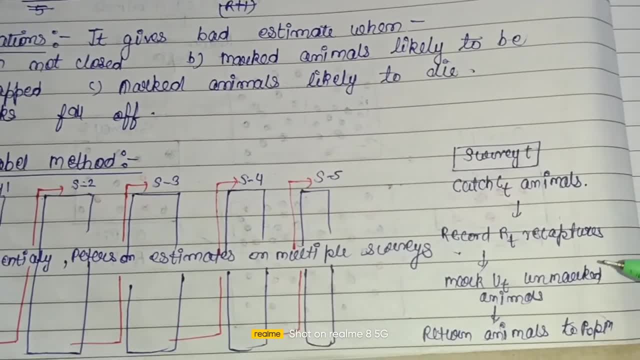 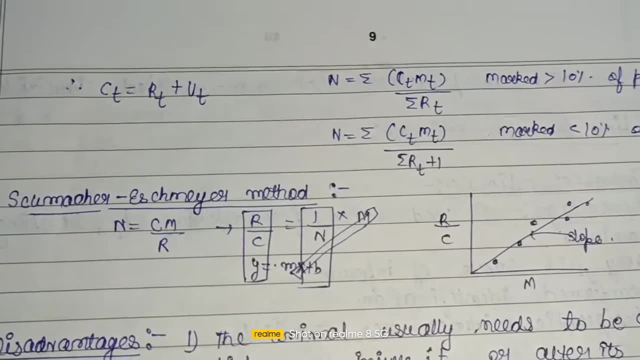 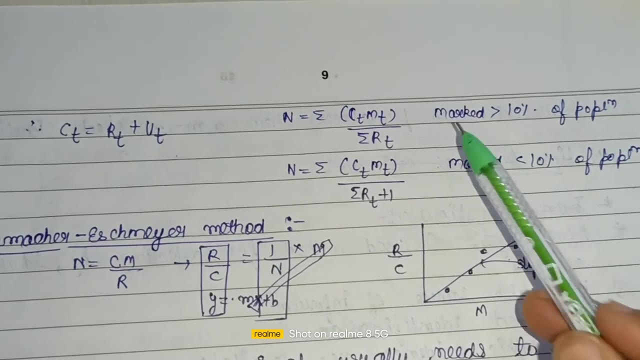 that if certain animals were unmarked, remain they are unmarked, then they should be marked and return the animals to the original population. so this is the formula ct, rt plus ut. this is also a formula, but you, you. but this is just for basic understanding. it is not important for the exam point of view. 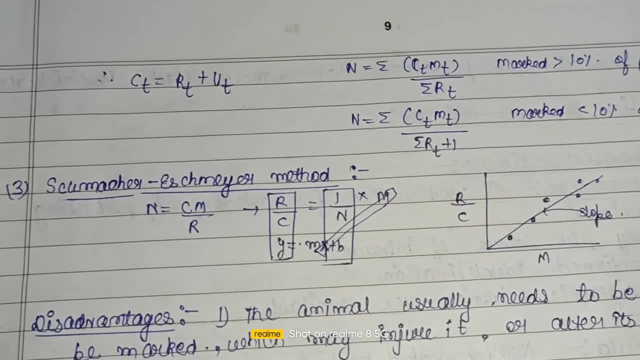 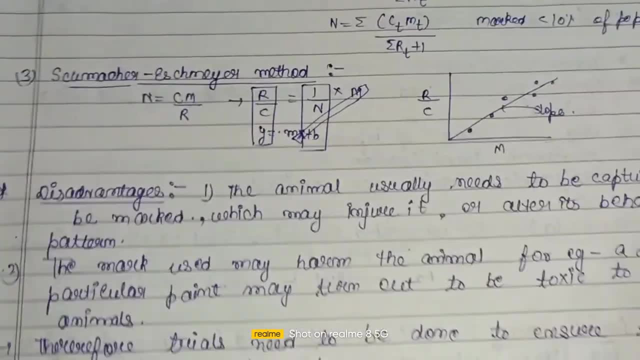 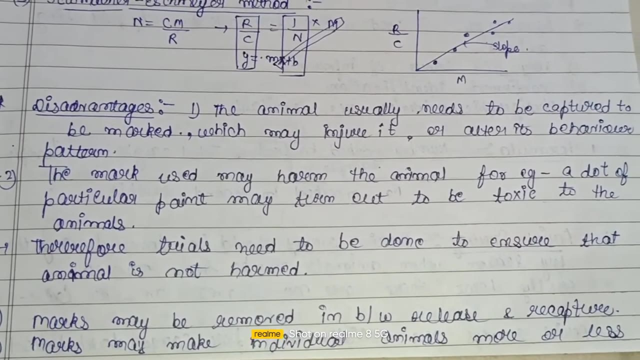 then the skew matcher, escamere method. so here also the formula is: n is equal to cm, upon my r that are that represent the recapture. okay, so these are advantages of this method. so the animal usually needs to be captured to be marked, which may injure it or alter its. 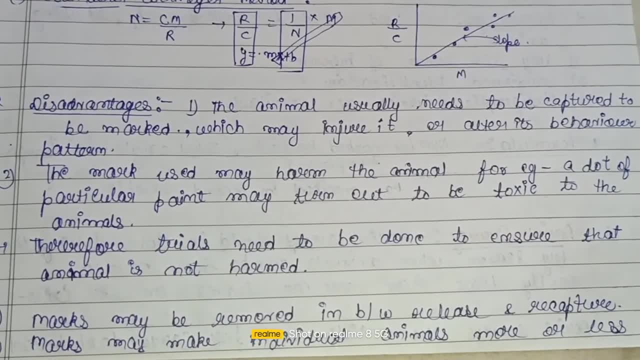 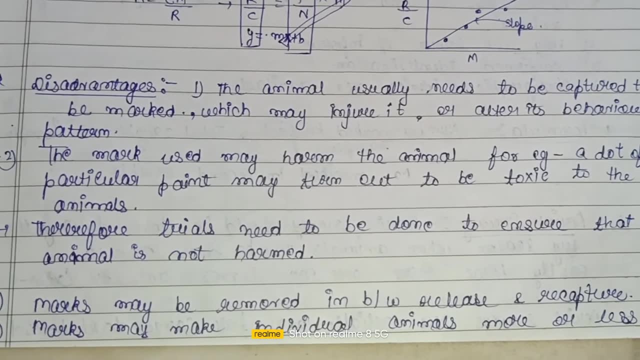 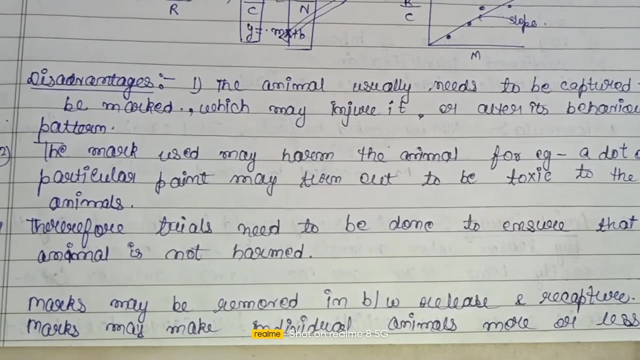 behavior pattern. second, the marks used may harm the animal. for example, a dot of a particular paint may turn out to be toxic to the animal. then, therefore, trials need to be done to ensure that the animal is not harmed. marks may be removed in between the release and recapture process.